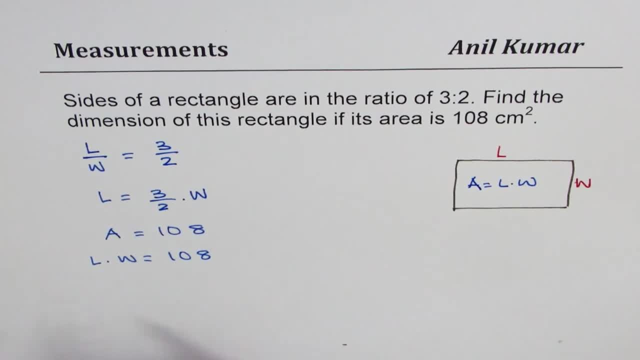 length times. width is hundred and eight. we can always write length as three over two times weirdly, so instead of writing length into width will replace L by three over two, w right times. we already have w equals to 108 and that gives you an equation which: 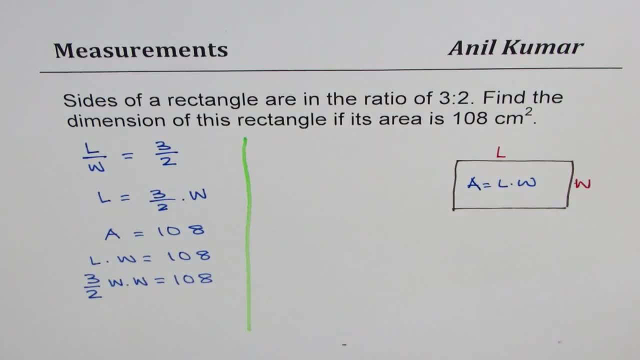 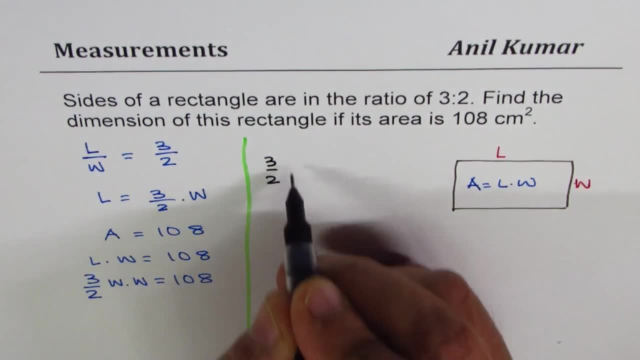 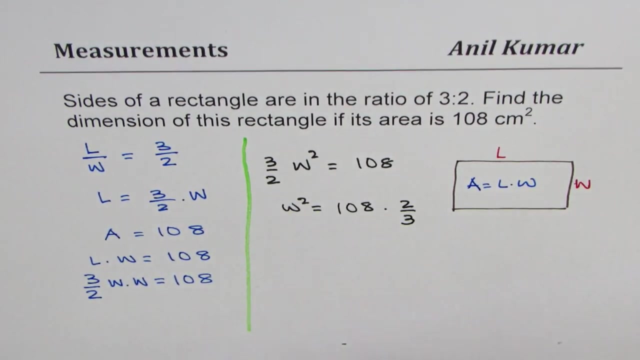 has only one variable, which is w which we can calculate correct. let me rewrite this equation here. so we have three over two w time, w is w square equals to 108, so w square can be written as 108 times 2 over 3, so cross multiply. this can be simplified: 108 divided. 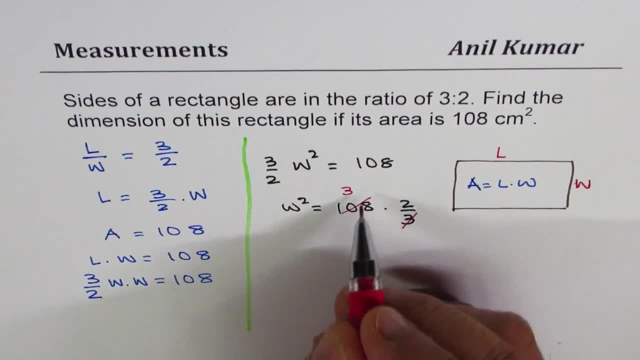 by 33 times 3 is 918. 3 times 6 is 18, correct. so that gives you, with w, equals to square root of this right. so we have 36 times 2, which is 72. so we have a square root of this. so we have 36 times 2, which is 72, so we have. 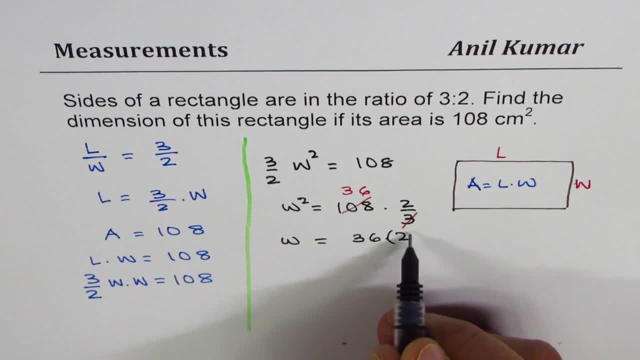 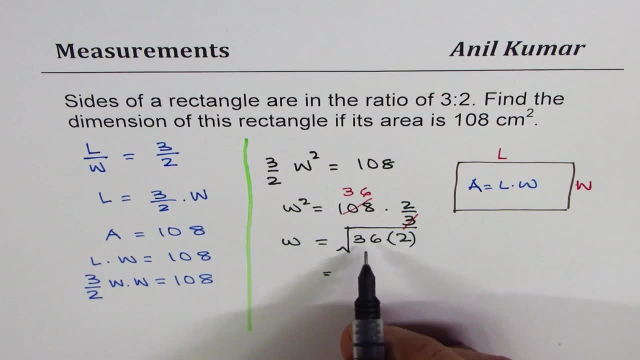 let's write 36 times 2. that's like multiplication and this is square, so it will be square root. so when you square root it, square root of 36 is 6, so we write this as 6 square root 2, so that becomes the width. now, if width is 6, 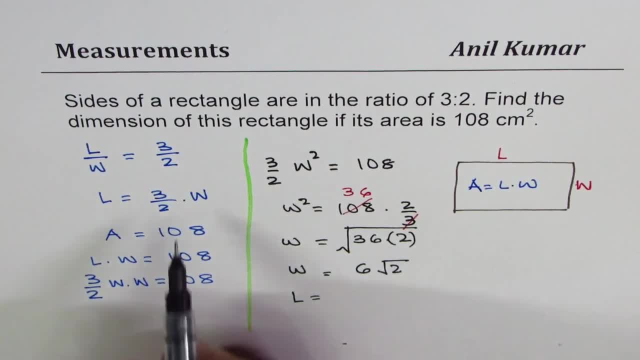 square root 2, length will be how much you can write. length equals to 3 over 2 of width, which is 6 times square root 2. right now, dividing this, we get. we could simplify this multiplying this by 3, so length will be equal to 3 times 3- 9. 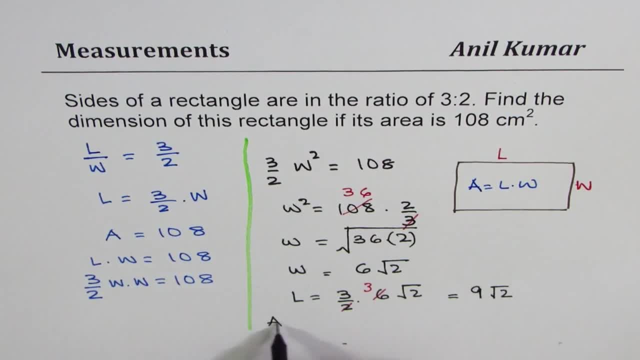 square root 2. so in this case, the answer will be that the dimensions are 9 square root 2 centimeters, since the area is in centimeter square by 6 square root 2 centimeters. correct? so that is how you can solve such a question. I hope it. 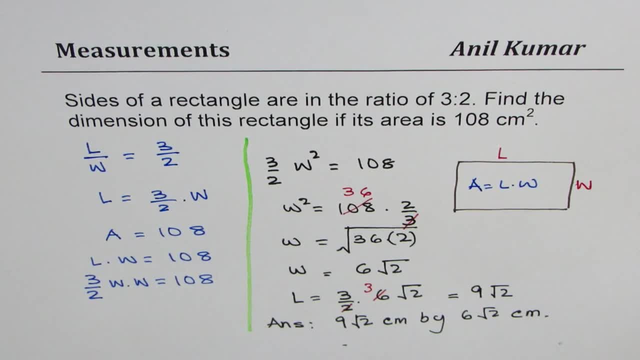 helps. thanks for watching. feel free to share my videos and subscribe to them. thank you and all the best.